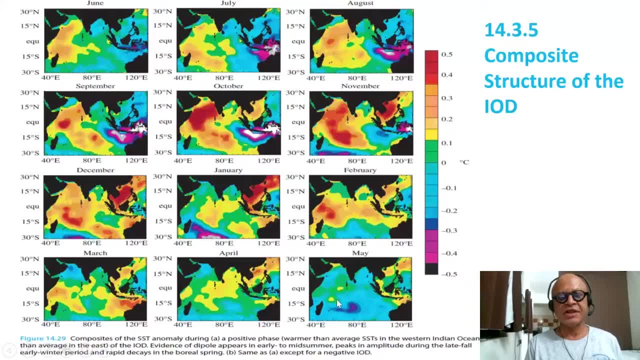 wide warming and then that dissipates into next May. So these are just shown as composites but honestly, most of the action happens here in these months and there is some evidence that the process may be initiated by air-sea interactions on this side related to the precipitation variability on this side, which itself could be related to this West Pacific maritime continent. So let's see that in a minute, but right now you can see that the cooling has peaked and disappeared, The warming on this side begins to take off and then by December you have essentially a basin wide warming and then that dissipates into next May. So these are just shown as composites but honestly, most of the action happens here in this region which is directly related to this West Pacific maritime continent. 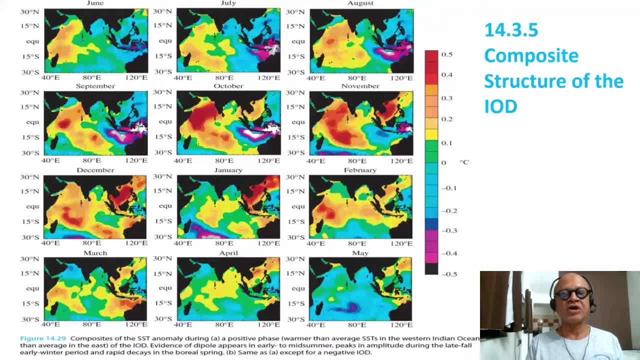 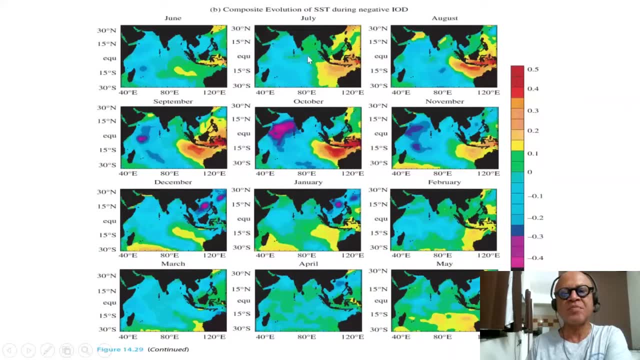 Convection complex, which is often referred to as the boiler box and so on and so forth, which has huge amounts of rain. The negative IODs is when there is a warming in the east and cooling in the west, so that also has an evolution in the same region, expands out into the southeastern Indian Ocean, grows in amplitude, and then you can see that the pattern is not exactly a dipole. This is why there is a debate and then the 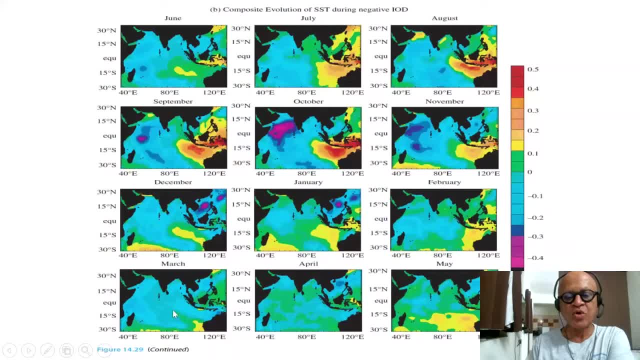 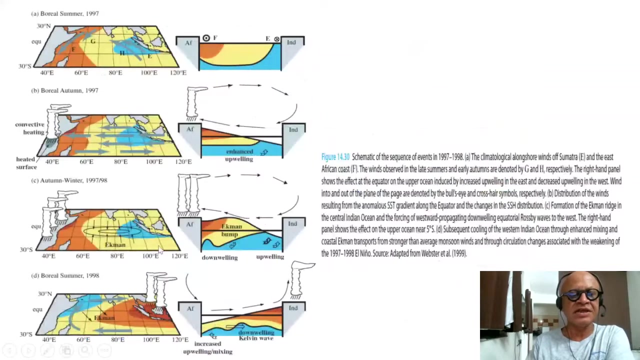 event disappears and then you get monopole across the Indian Ocean. So this debate will go on: Many unanswered questions about the dynamics and thermodynamics and, of course, El Nino is studied for so long with so much data and we haven't answered many questions, so you can imagine that this is going to take some time. This is the idea of evolution of the 97-98 event from this Webster et al fable, from 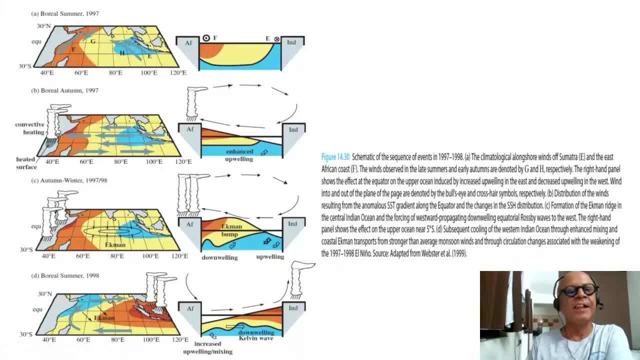 1999, which talks about the beginning of the alongshore winds, which I said is potentially related to the Indonesian rainfall anomaly over here, and then, associated with that, there is a thermocline signature in the ocean that grows into this easterly wind anomalies, convection on this side and then a stronger east-west tilt of the thermocline, like in the. 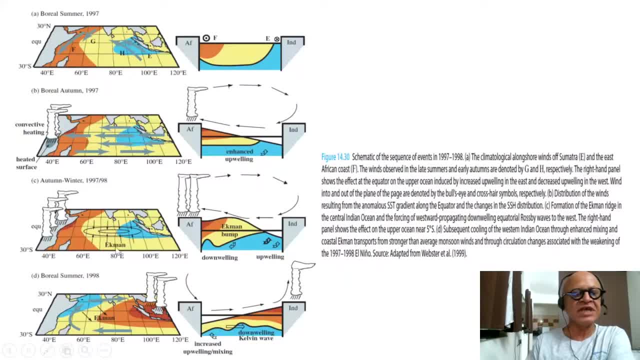 Pacific, except that it's in the opposite sense. and then you have all these nice Ekman processes that begin to turn the process around, and by the boreal summer of 98, it's not clear. the life cycle is really that long. Seems like things disappear by December of 1997 itself, So September-October. 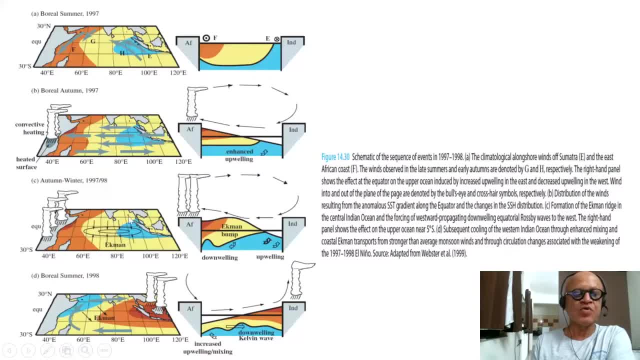 November of 97 the cooling is peaked, and then December 97, the basin-wide warming is already in place, which is very similar to what you expect in the Indian Ocean during El Nino years as a teleconnection. and then there is something called the Indo-Pacific capacitor, where the delayed warming over the Indian Ocean has an impact back on the Pacific, and so on. 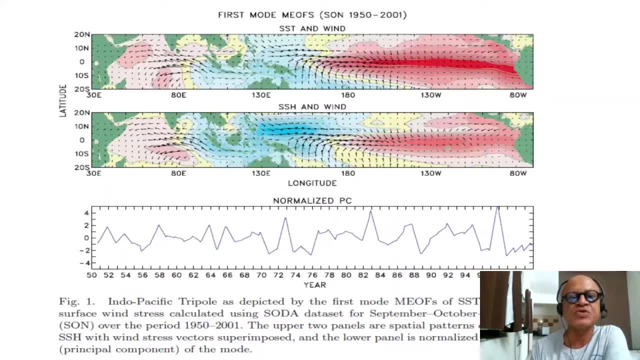 So leaving that as it is, I know I kind of rushed through it because I think that story is given a lot of space in the book but a lot of the new literature is not included. So the idea from Doc Chen which has been proposed is that there is actually something like a tripole in the Indian Ocean. So this really depends on how you analyze. We have looked at El Nino and talked about Nino 3.4, Nino 4, Nino 3 and so on. 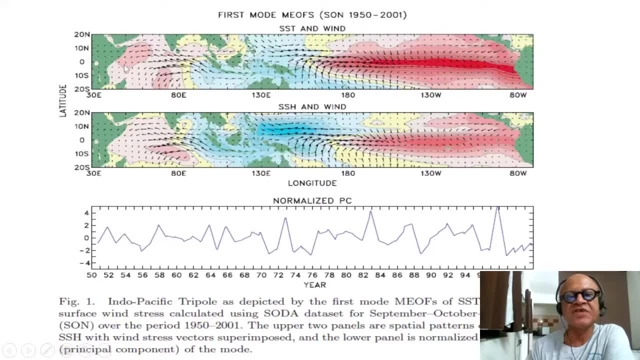 But you do the analysis over the Indo-Pacific, then you get a better sense that the Indo-Pacific warm pool has a coherent anomaly here with the divergence around the maritime continent and the Indian Ocean response is like the dipole, which we have been looking at just as an Indian Ocean phenomenon. 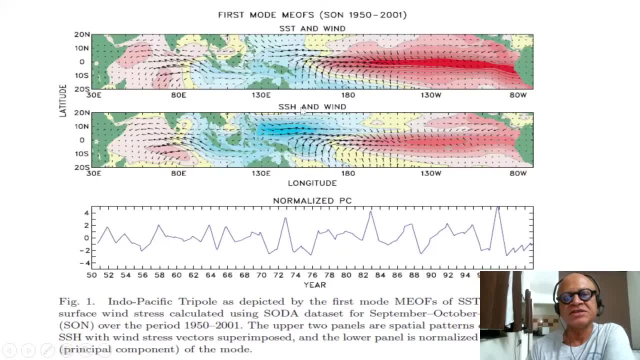 So that's in SST and winds and this is in sea surface height and winds. So you can see all kinds of signatures that are consistent with the El Nino here and the Indian Ocean dipole here. And if you do the normalized PC, these are the empirical orthogonal functions and if you look at the time series or the principal component associated with that, you do get the El Ninos and you get the IODs and so on. 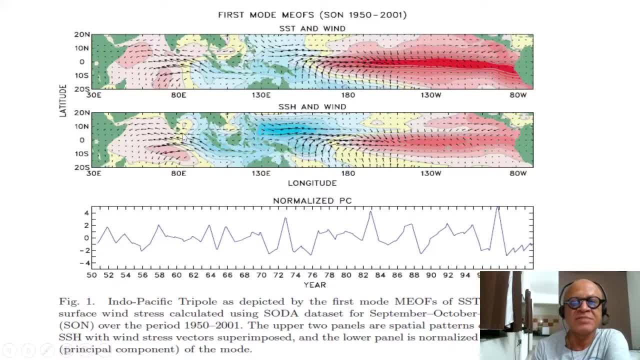 So is it that the Indian Ocean is back on the Pacific? Yes, the Indian Ocean is basically a close partner of the Pacific Ocean, and that they are really not able to vary so independently. It's this big heat source that can force both oceans more directly here through the oceanic tunnel, the Kelvin waves and the thermoplane signal, the delayed oscillator, recharge, discharge, and so on. 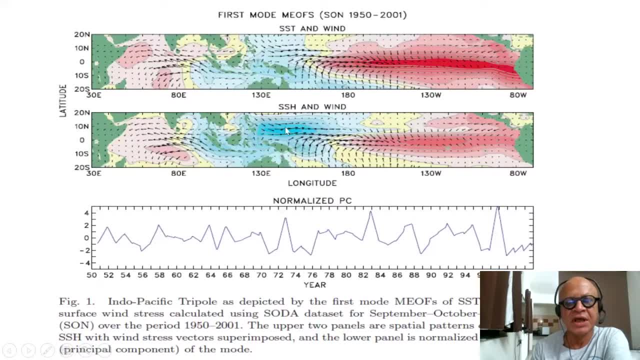 Whereas on this side it's a combination of the atmospheric bridge with the subsidence on this side, Rossby waves along shore, winds and maybe an oceanic tunnel through the so-called Indonesian through flow, which we haven't talked about much. So this is really an open question. 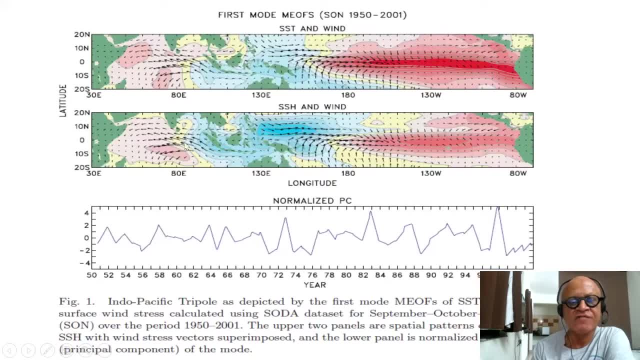 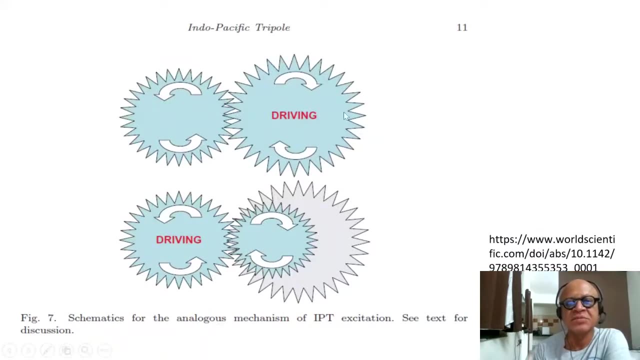 So in the end it may turn out that the strong influence of the Indian Ocean on the Pacific and the IOD may be part of this kind of Indo-Pacific tripole. And Doc Chen kind of puts it in this perspective where he says the Pacific is the big gear. 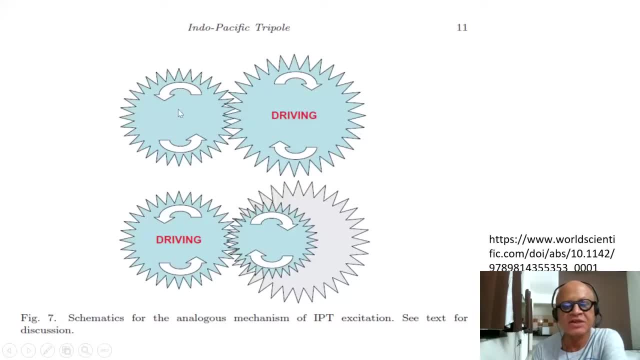 And the Pacific is the big gear And the Indian Ocean is the small gear, So the big driver is controlling most of the time, but sometimes the Indian Ocean is able to be the driver. So this may also explain why 50% of the wet and dry years are not really explained by El Niños and La Niñas. 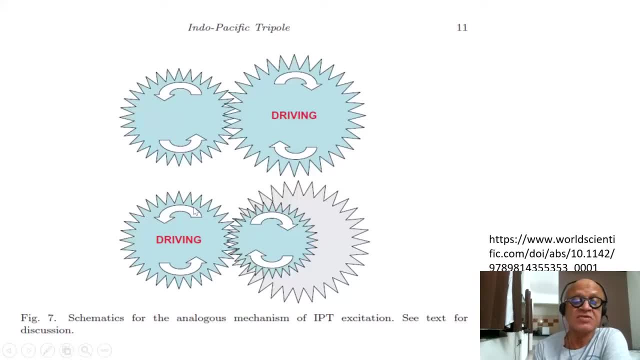 Because, considering that the monsoon itself is a big heat source as well, we have to understand how it is that the interactivity between the two oceans is so important. So this is a big question: The interactive system of the monsoon and so Indian Ocean, etc. can work together. 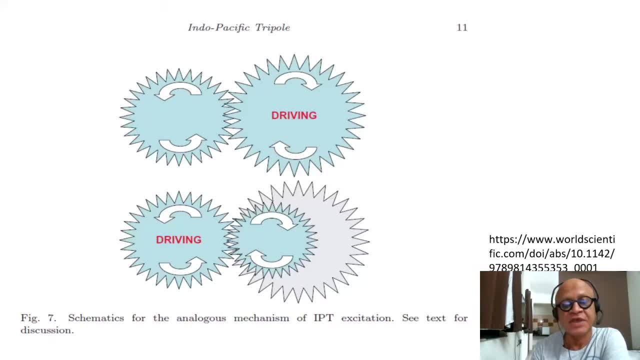 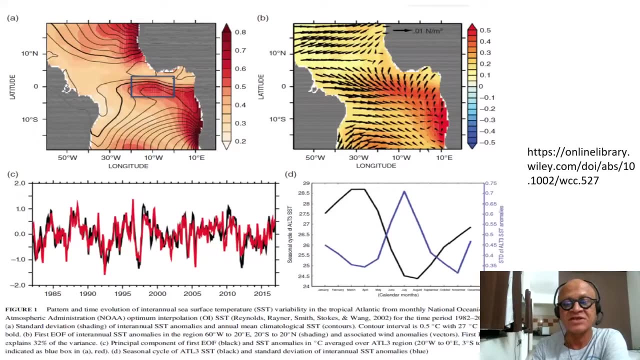 So this is something that I would consider somewhat of an open question. that needs some new ideas, because we are basically struggling with the older ideas. Just to close out the chapter, then the Atlantic Ocean also has something like an El Niño mode. It's called the Atlantic Zonal Mode or the Atlantic Niño. 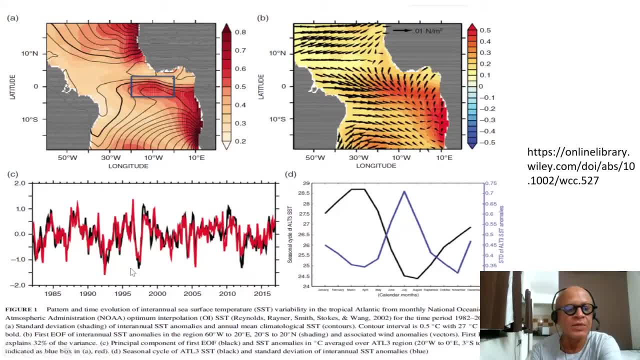 And this is showing the pattern and time evolution of the inter-annual sea surface temperature variability in the tropical Atlantic from the NOAA data. And this is the region which gets warm. It doesn't have as much of a strong zonal contrast as the Pacific. 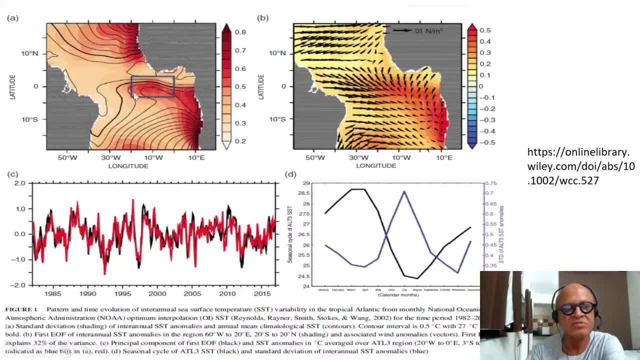 And the zonal extent is small, so the wave travel times are small. And because of this Gulf of Guinea, here the upwelling signal is also a little bit different than the cold times And because the ITCZ is sitting across like this and the boreal spring ends up touching the equator. 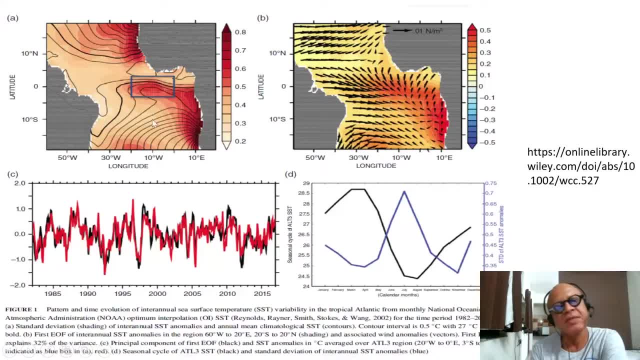 there is a strong relation between the meridional mode of variability and the zonal mode of variability, But nonetheless, when you look at the composites you get a sense that they are pretty close to each other. So here you are seeing the principal component of the first equation. 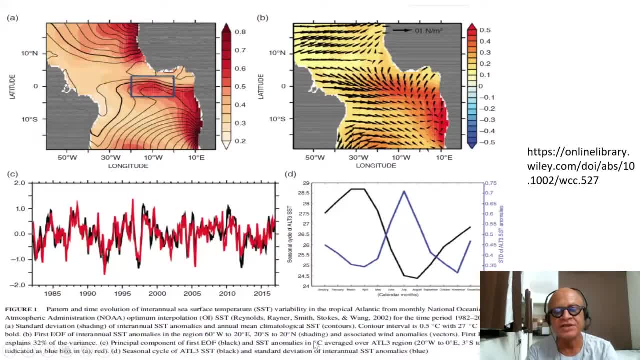 We have the first EOF and SST anomalies, So they both are highly correlated. as you can expect, There is an Atlantic III region where SST anomalies are created, like the Niño III index. This is called the ATL III index And this is the seasonal cycle of the ATL III box. 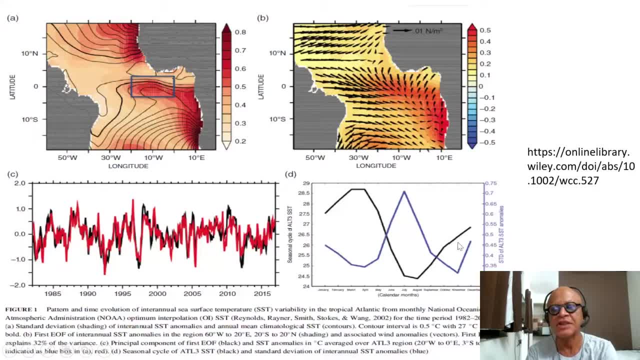 and standard deviation of the intra-annual sea surface temperature. So you can see that when the summer months come, the seasonal cycle of the Atlantic SST gets weak but the variability goes up. So whereas the Indian Ocean Dipole peaks in September, October, November, the Atlantic Niño III is peaking in July, August, September And that has an impact on the monsoon. So maybe some of the unexplained or non-El Niño droughts and non-La Niña floods may be related to the cold and warm events in the Atlantic Ocean. 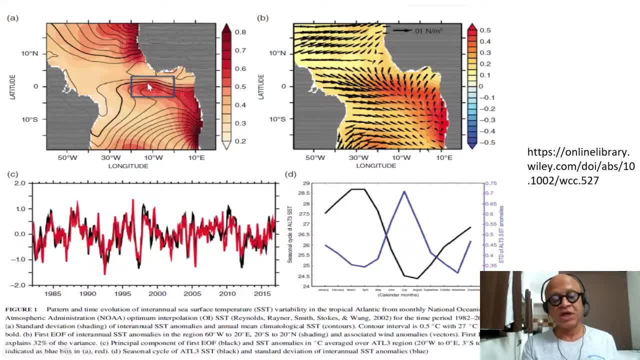 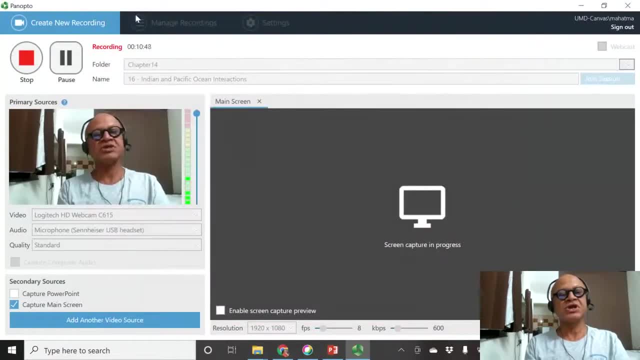 There is a lot of literature on the Atlantic Niño as well, which we haven't gone through, but there are some commonalities in the processes: recharge-discharge, biechnitz, feedback and so on. So if I have to give you one point of view, 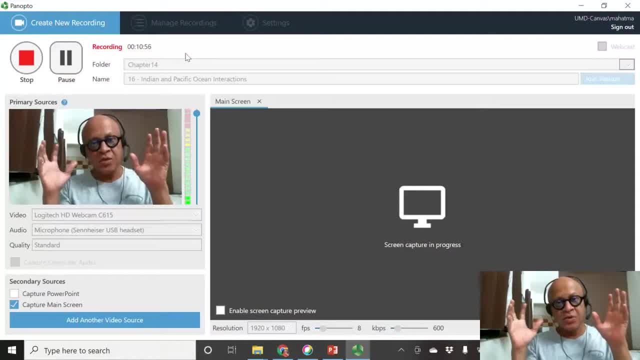 it would be that the Indonesian region and the West Pacific warm pool generally has a huge heat source in terms of that convection And when that jiggles it can set off these zonal disturbances and maybe all the eastern ocean responses in the Atlantic, Indian and the Pacific.